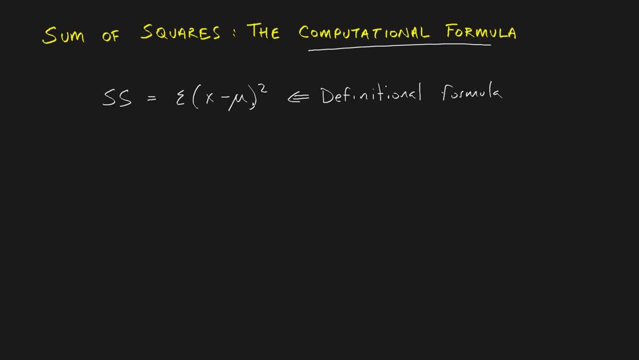 positives and give us a zero as an answer. So we took our deviations from the mean, we squared them and then we sum them up. Why did we sum them up? We sum them up? because we're looking for an average deviation Or what we, what my videos have shown so far, what? 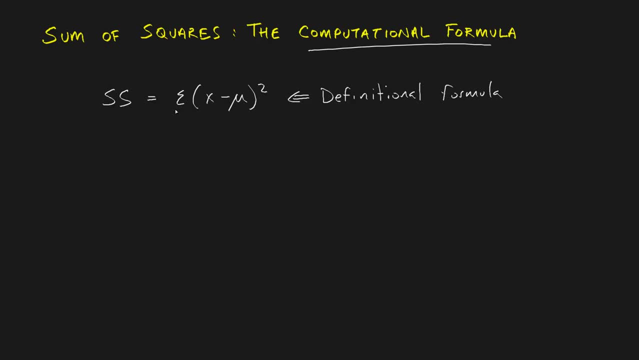 we call a standard deviation. It's trying to be an average deviation. It's on average. how much do scores deviate from the mean? Well, any time you're going to take an average, you have to have a sum over the number of things that went into that sum. You 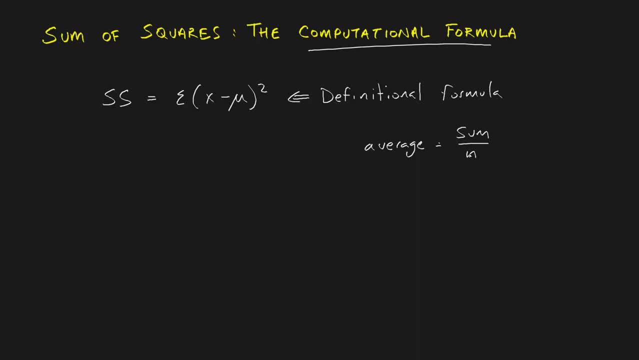 have a total over the number of things, that are, the number of things that contribute to the total. So that's what an average is, or a standard. A standard deviation is like an average deviation, Alright, so that's what we've done so far. The new formula that I'm introducing. 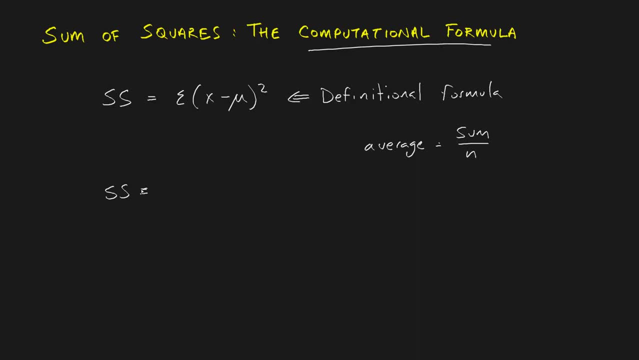 here is called the computational formula. Now, it's called a computational formula because it's a little bit easier to work with in terms of the number of things that went into that sum, In terms of actually crunching numbers, If I have a big list of data, if I have a large sample. 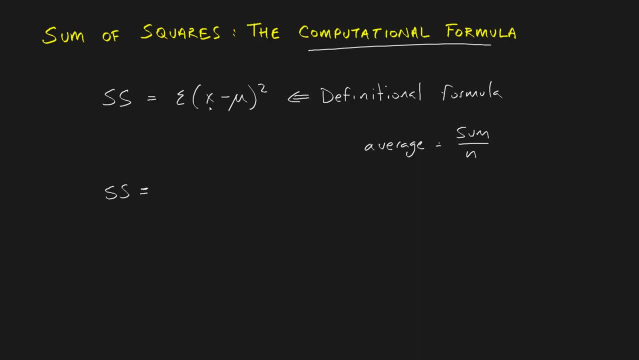 I might not want to have to go through and find every single deviation first and then square them and then sum them up. This formula is actually going to look a little bit worse. It seems like there's more going on here, but it's a little bit easier to work with when you have a lot of data. Okay, so this is the. 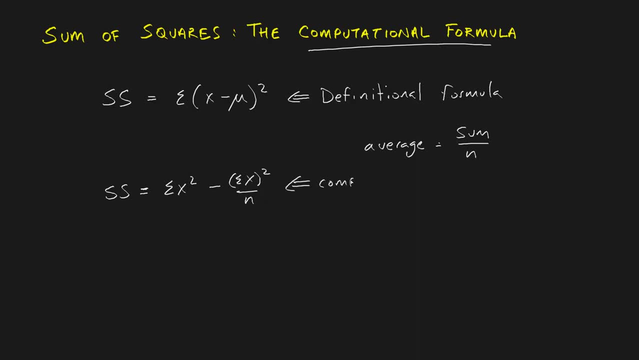 formula. This is what's called the computational formula. Alright, I think the best way to illustrate this is to just show you both formulas being used side by side. So I'm going to set up some data here. Let's work with some values. 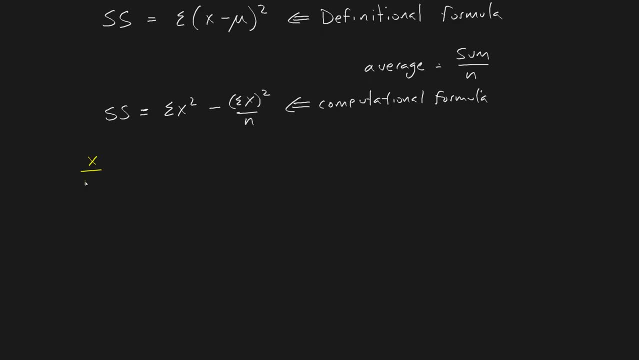 that we've been working with in some other examples. So I'm going to work with 48, with my data being 48, 49, 50, 51 and 52. you might recognize this from a previous concept video where I found that the total was equals to 250 and I 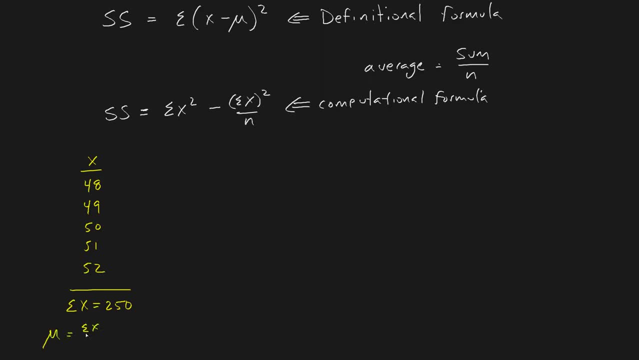 use that total to find the mean, that is, 250, or, sorry, the sum of X over n, which is 250 over 5. my average is 50. so if I want to use the definitional formula, if I want to show you the definitional formula, the first thing that I do- 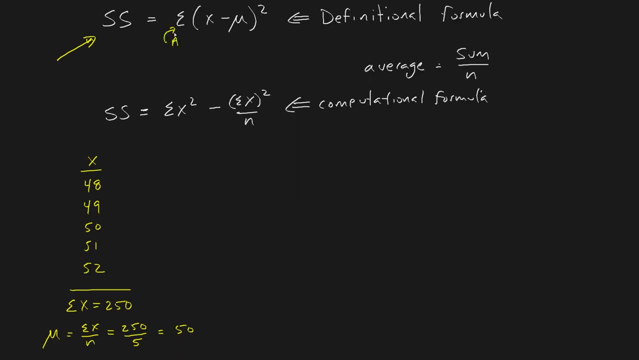 considering that I have addition. that's what a summation sign is telling me to work with. I have brackets, I have subtraction and I have an exponent. the first thing that I need to do is deal with the brackets, because order of operations or bed mass tells me I start. 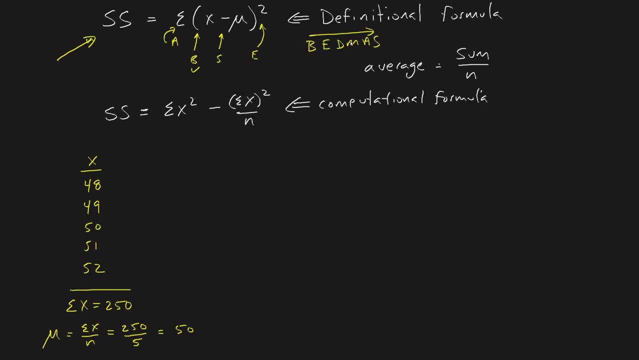 with brackets and work my way through exponents, division, then multiplication, then addition and finally subtraction. now we have subtraction inside of our brackets but because we have to do brackets first, I'm going to work out that subtraction in my first step dealing with this data. so I'm gonna do. 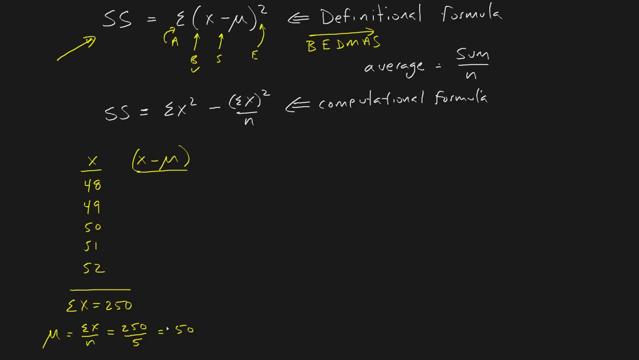 icked. look at what I've put in to my table and I'll give you a call back from someone, and the next thing that I'm going to do is look at my total. so what I need is the subtraction side of those brackets with brackets I'm going to take. 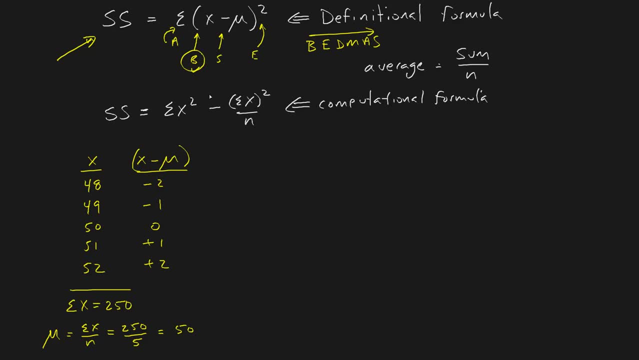 the second fraction of all these exponents I brother in trigonometric ante front, one to the right. so it ser Tri section that first of all this subtraction is going to be the sum of the uppercase left over. so that's only the 90 per second in this picture, or only the value of 1. this algebraic will be this: 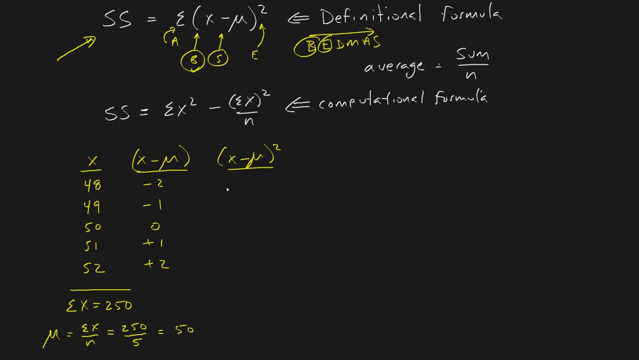 results, square them. All of this is stuff I've done in previous videos, So this is just sort of a recap of the definitional formula. I have to square each of these results. So negative two squared is four, negative one squared is one, and so on, And so that takes care of my exponents. 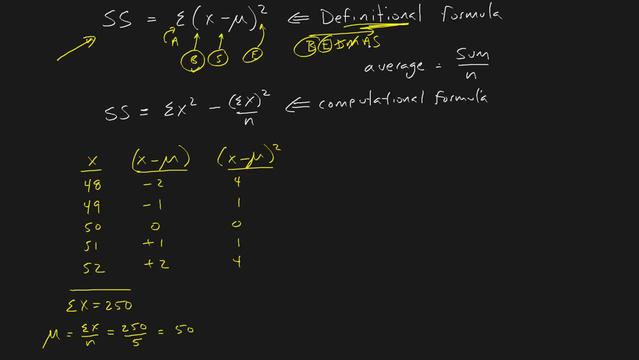 There is no division, there's no multiplication, but there is addition. So that's the last thing that I do. I have to add these up, And so when you add them up, you get four plus one is five plus one is six. 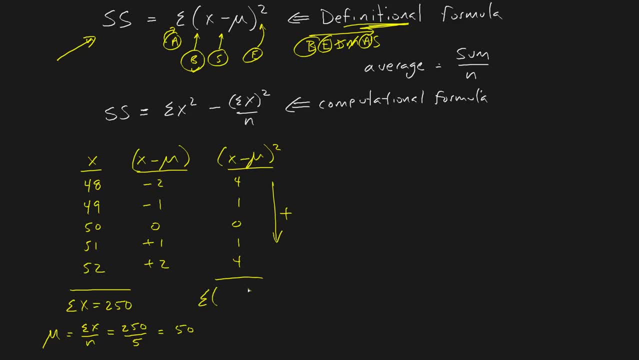 plus four is ten. So I've now summed my squared deviations And that gives me ten. So my sum of squares is ten. So that's done. But what if I do the computational formula? Well, I'll start with the same data. 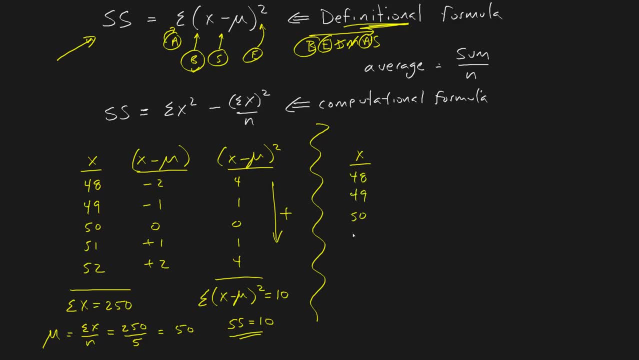 But imagine that I hadn't done anything yet, I just had my data. Last time I had to add up all of my data. The sum of x is 250.. Do I need to do that again? Yes, I do need the sum of x, you can see. 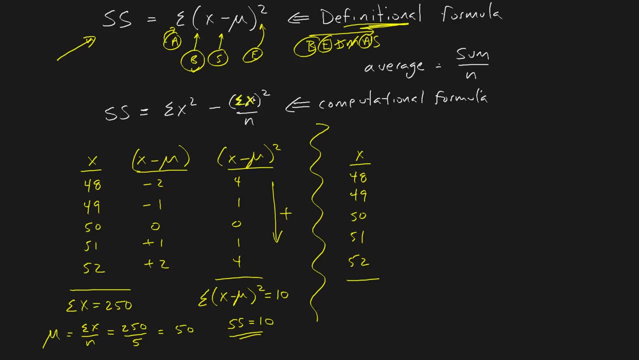 it's right. here There's the sum of x. So I work out that the sum of x is equals to 250.. Now, the last time I used the sum of x, I had to add up all of my data. So I had to add up all of my data. The sum of x is 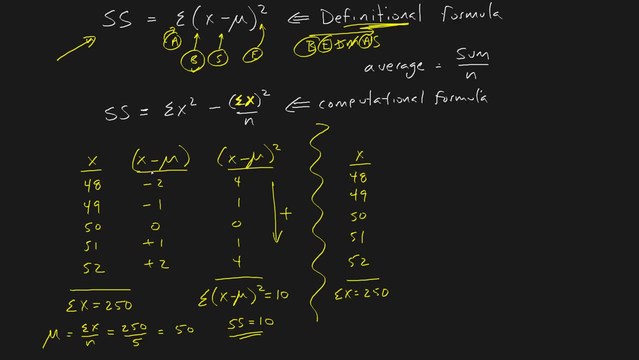 five. So I'm going to use that to find the mean, because I needed the mean to find deviations. When I'm dealing with a computational formula, though, I don't need to find a deviation. I don't need to find the mean. it doesn't exist in the formula at all, So I'm not going to bother with that. In fact, the only thing 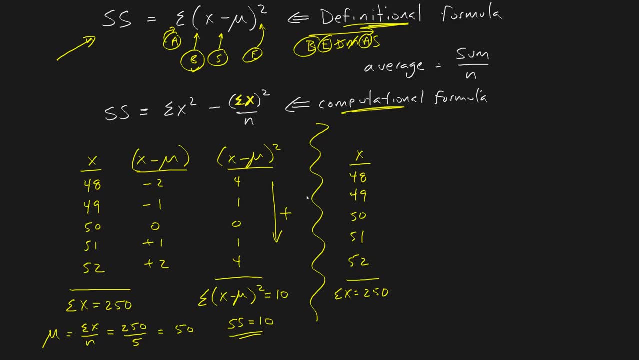 that I need, or the only things that I need, are the sum of x, which I've already done. I need n. well, n is simple. it's just one, two, three, four, five different values. So I know that n is equals to five. 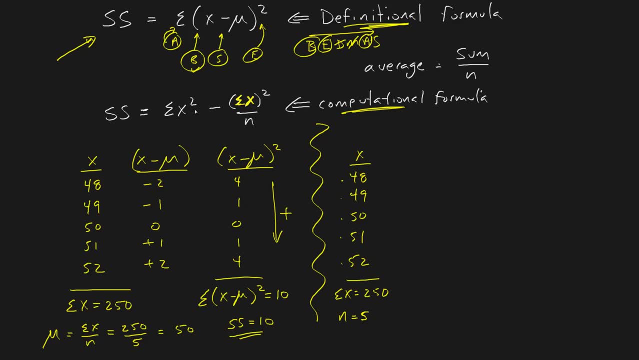 And finally, I need to know the sum of x squared. Well, now, this one you have to be careful about, just like up here where we did order of operations, to figure out which order to perform all these operations in. When I have the sum of x squared, I've got two things going on. I've got summation. 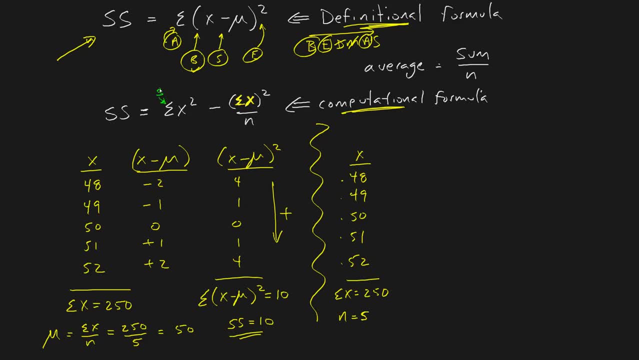 that's addition. sorry, I guess I should call that. don't want to confuse it with subtraction, So I'll call that a for addition. That's what summation is. So I'm going to call that a for addition. That's what summation is. So I'm going to call that a for addition. That's what summation. 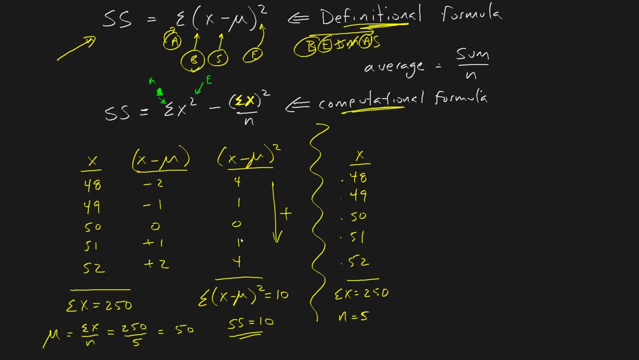 is, And then I've got an exponent going on there. If I'm looking at order of operations, there's no brackets but there is an exponent, So that's going to come next or that's going to come first. So I 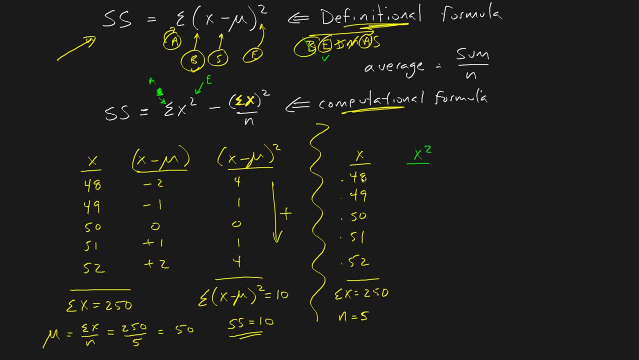 have to square each x. So I have to do 48 squared, and then 49 squared, and then 50 squared, and so on. So 48 squared is 2304.. 49 squared is 2401.. 50 squared is 2500.. 51 squared is 2601.. And 52 squared is 2704.. Now I don't just need x squared. we've done the. 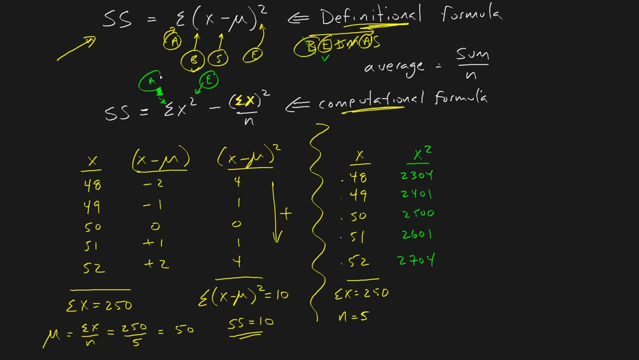 exponents. we need to now take care of the other operation. here we need addition. we need to add these up. that'll give me the sum of x squared, And when you add up all five of these values comes out to be: 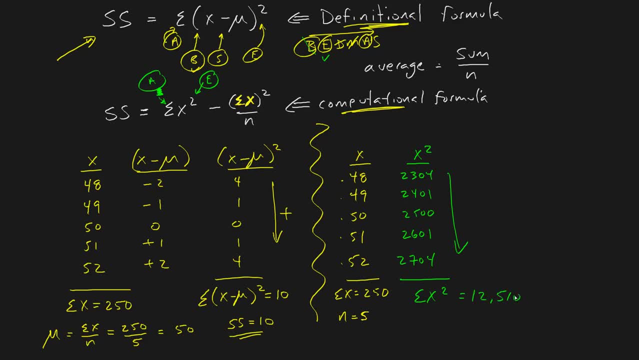 exactly 12,510.. Now what I can do is I can plug each of these values. I've got my sum of x squared worked out, I've got my sum of x worked out, which I can square, and I've got n, So I'm going to work all of. 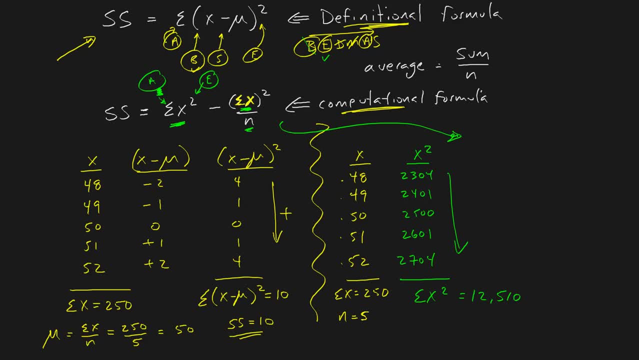 these into the formula. Sum of squares equals to the sum of x. squared that one is 1250, or, sorry, 12,510.. Minus the sum of x in brackets, which is 250.. Square that and divide by n. 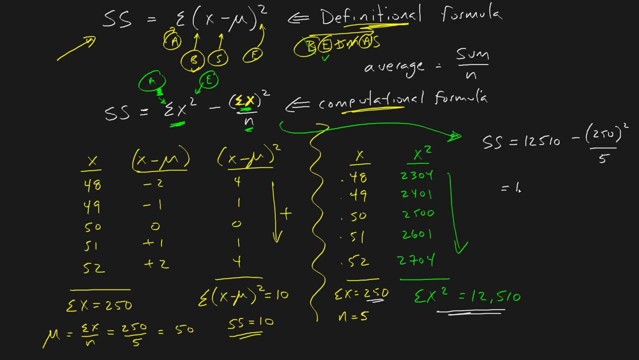 which is five. So let's do the fraction first. This is 250, squared is 62,500.. And we're going to divide that by five, And so this ends up being 12,510, minus this fraction. When you work this out, it comes out to be 12,000, even. 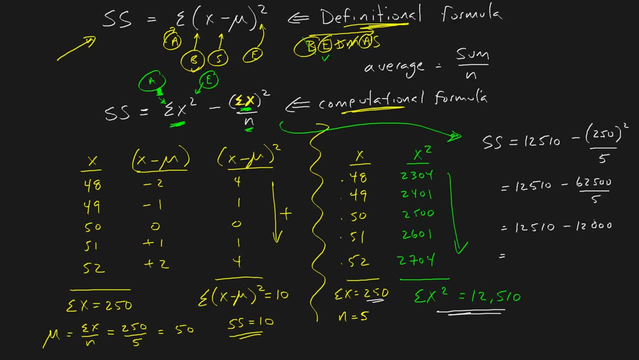 And so we end up getting- or sorry, 12,500.. Let me correct that here. And so the answer ends up being 10.. So the sum of squares is 10.. This is the same as what we got when we did the definitional formula. 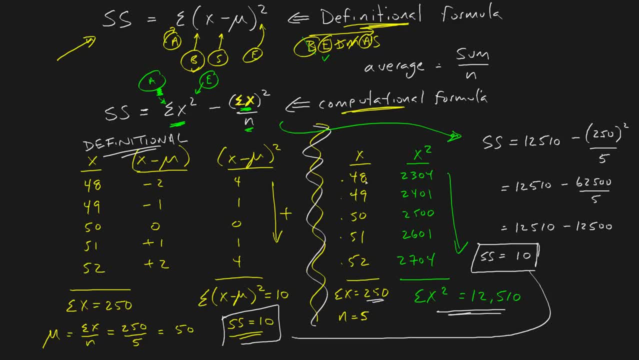 Over here, on this side of the squiggly line, we have the computational. Now, remember what I said was that the computational is used, or its reason for existing is, to allow you to do less, When we were dealing with the definitional formula. 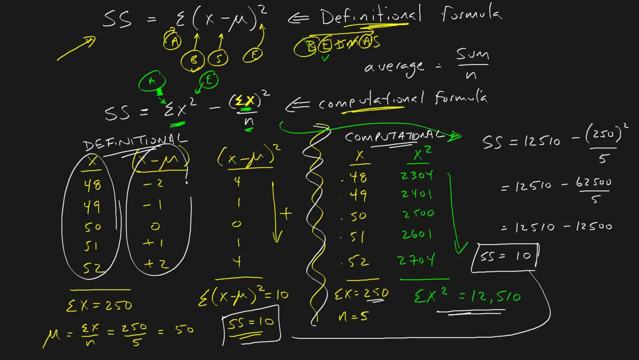 we had to work with our raw data, Then we had to find deviations, Then we needed a third column to square the deviations With computational also. actually we had to work out the mean With computational. we had our raw data which we added up. 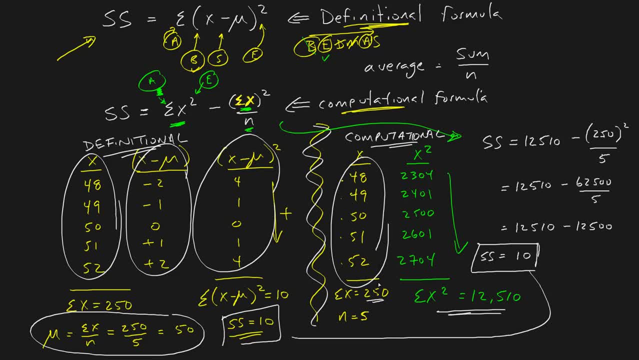 But we didn't have to find the mean and we didn't find deviations. We just had one other column And then we jumped right into finding, or we jumped right into substantiating, We substituted things into our sum-of-squares formula. 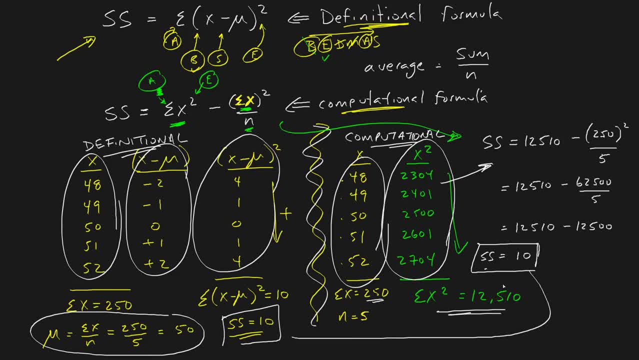 So it was a little bit less work. We only had five data points, though If we had a lot of data, if we had 100 data points or 1,000 data points or something like that, it would have been a lot less work to use the computational formula. 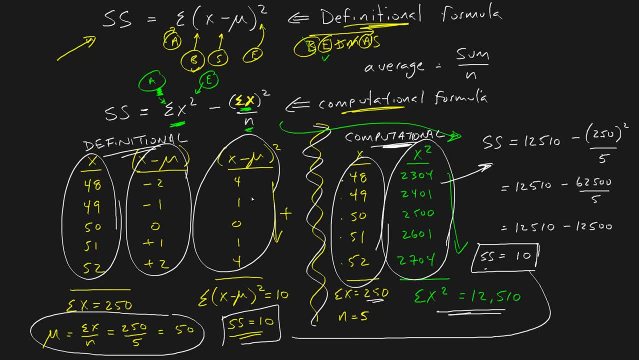 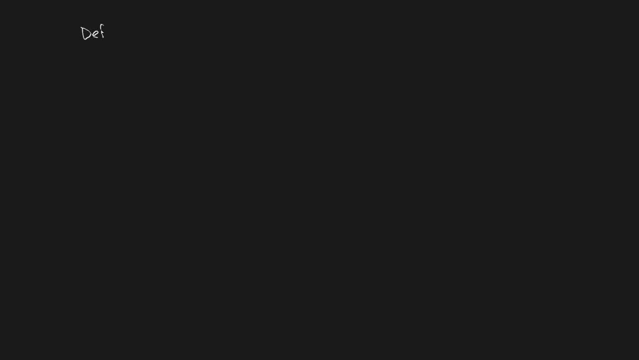 So this formula, this second formula- let me just put these side-by-side again. The definitional formula is: sum-of-squares is equals to the sum of the squared deviations from the mean, And the computational is: the sum-of-squares is equals to the sum of x squared minus the sum of x in brackets, squared over n. 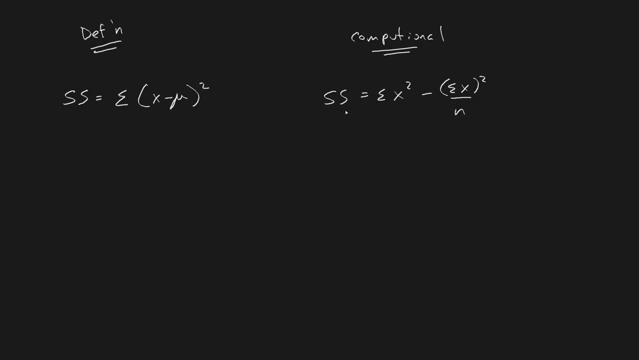 These two formulas will always produce the same result. If you are more comfortable with using one over the other, then go ahead, Unless they specifically say: use the computational formula to figure this out. but I doubt they're going to do anything like that. 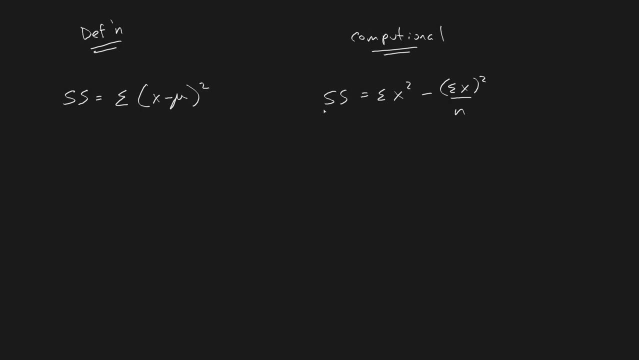 So you can use whichever one makes you more comfortable. They both will always give the same answers, regardless. It makes no difference which one you use. However, the computational is a little bit easier when you have more than a few data points, So you might want to get used to dealing with that.